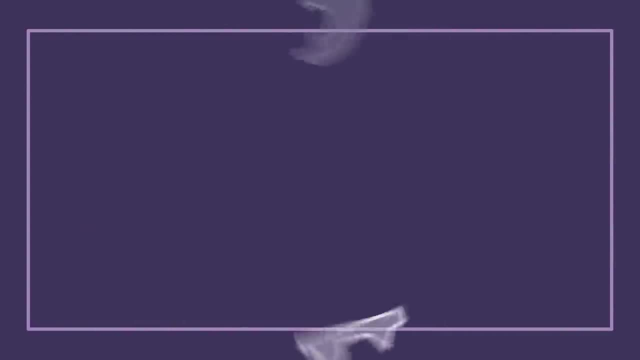 are always moving and occasionally they collide at the right speed and orientation so that the substrate fits into the enzyme at the active site. Collision theory dictates that collision must occur with sufficient energy and in a specific orientation for a reaction to occur. Enzymes are specialised. their active site matches the shape of a specific. 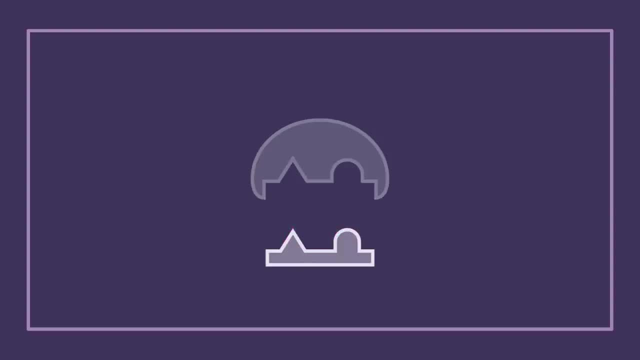 substrate that they can react with The enzymes, and the substrates fit together using a lock and key mechanism. Once the substrate is in the active site, the reaction takes place – the required product is produced and the enzyme releases itself and carries on moving around. In this example, the enzyme is breaking down. 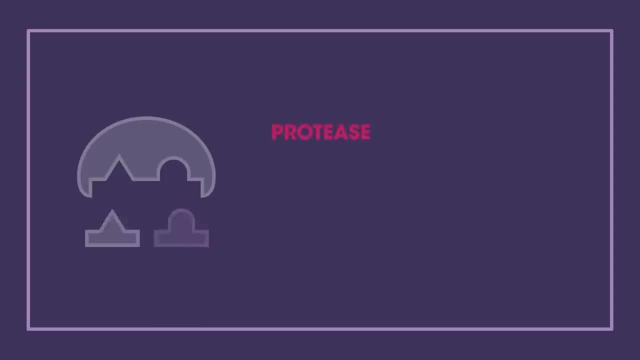 the substrate into two smaller products. It could be protease, which breaks down proteins into amino acids, or carbohydrates, which breaks down carbohydrates into glucose, or lipase, which breaks down fats into fatty acids and glycerols. Hydrogen peroxide is often formed as a result of the reactions in cells and, if it is left, 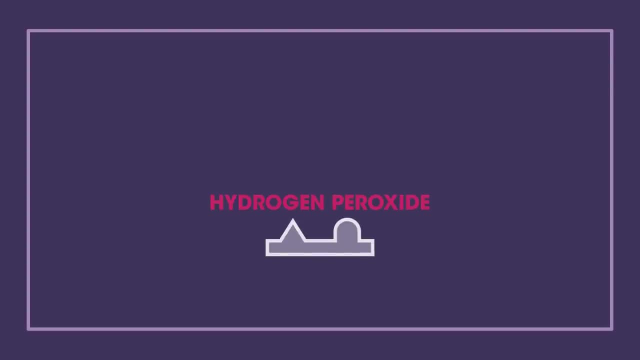 behind to build up. it is harmful. Luckily we have catalase enzymes that are really fast. They break the hydrogen peroxide down into harmless water, and oxygen Enzymes can help build up molecules like this, but the process is still exactly the same. 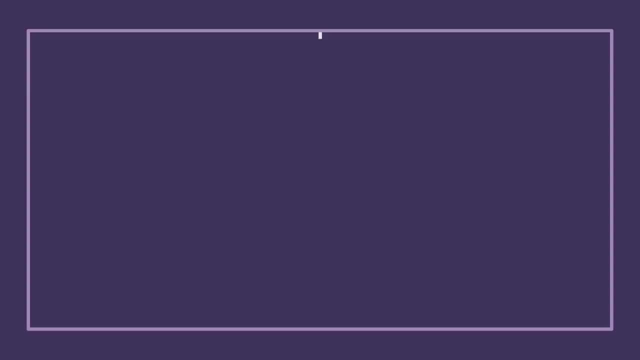 Whilst enzymes do fantastic things, they are sensitive. Each enzyme has optimum conditions under which it works best. Firstly, there needs to be enough substrate around. They need a high enough substrate concentration for the reaction that they catalyse. If there is too little substrate, then the rate of reaction is slowed Sometimes if there is, 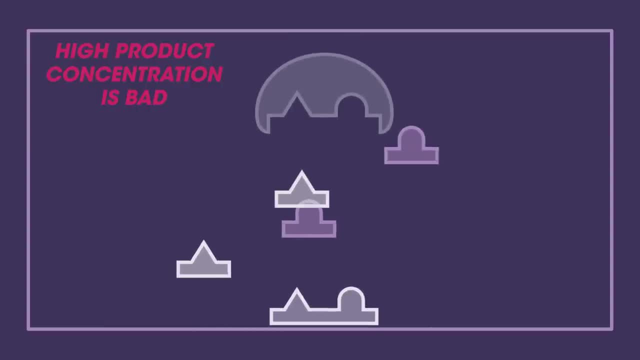 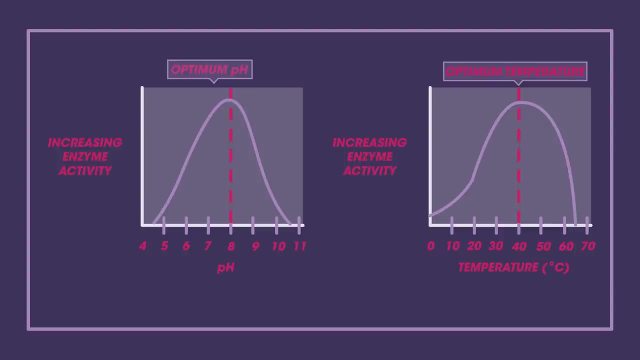 too much product around, then the reaction slows because the enzymes and substrates have less chance of bumping into each other, So the product needs to be removed. for a higher rate of reaction, Enzymes also have optimum pH and temperature conditions Up to a point. an increase in temperature causes increased rates of reaction. 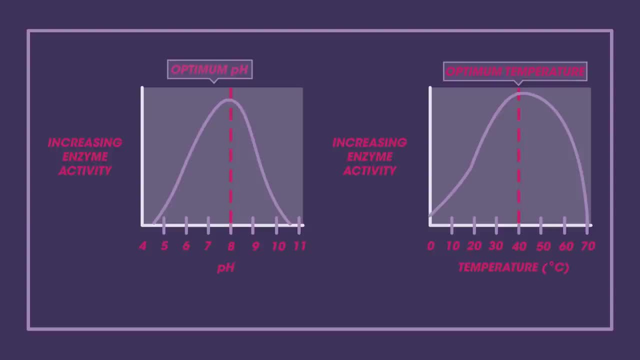 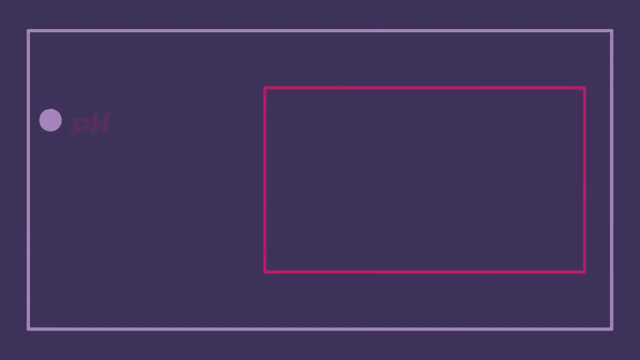 Because there is more heat energy. More energy means more collisions. However, above a certain temperature, the rate drops off due to denaturation. We will look at the effect of pH and temperature on enzymes in our video. Denaturation of Enzymes- The optimum pH and temperature conditions. 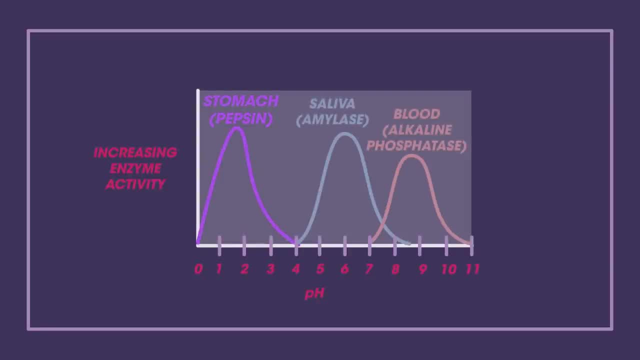 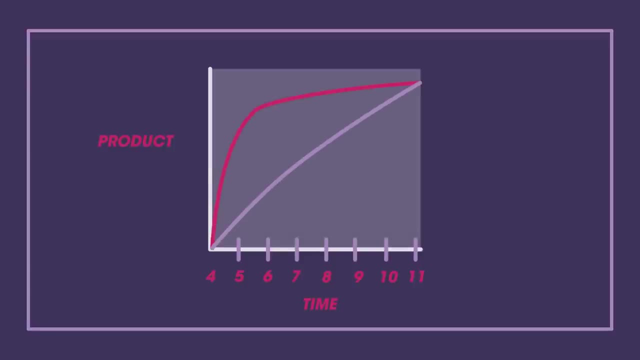 are specific to the condition in which they work. in An enzyme that works in the stomach, for example, would have a more acidic optimum pH, And of course there need to be enough enzymes around for the rate of reaction to be optimised.